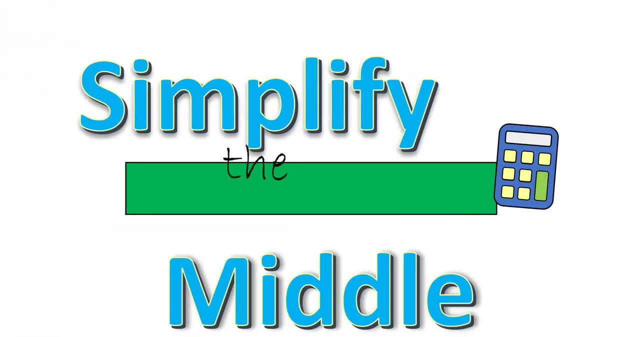 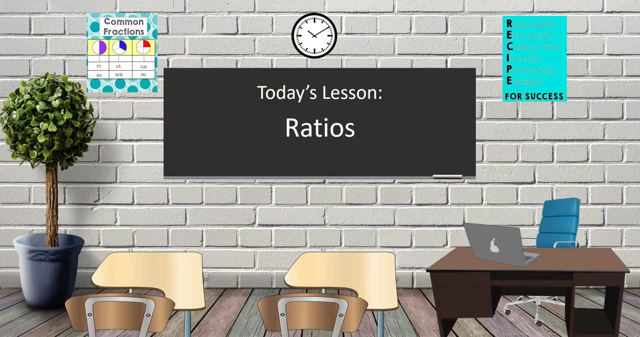 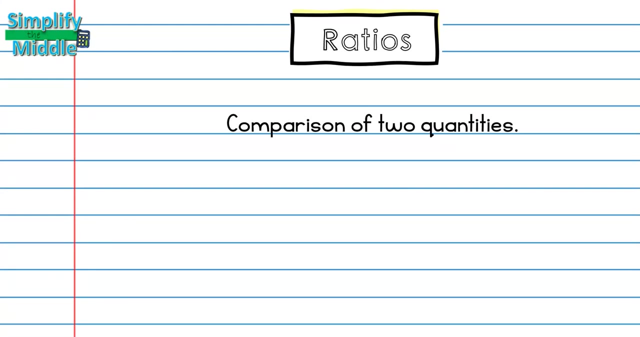 Hi and welcome to today's lesson: ratios. A ratio is defined as a comparison of two quantities. A quantity is an amount. Let's look at an example of a ratio. This question asks: what is the ratio of purple to green pencils? I can see that I have one purple and four green pencils. 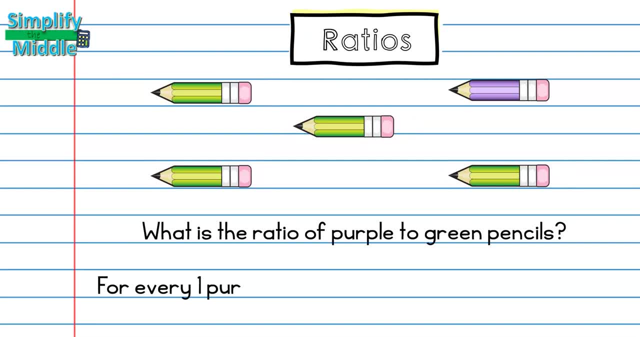 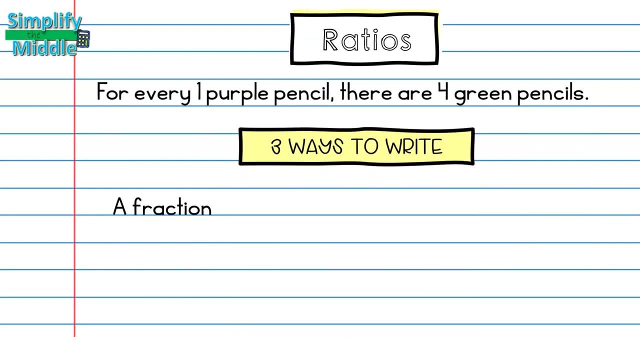 This means for every one purple pencil. there are four green pencils. Ratios can be written three different ways. We can write a ratio as a fraction, So in this case one over four. One is representing our numerator, which is purple, and four is our denominator, which is representing our. 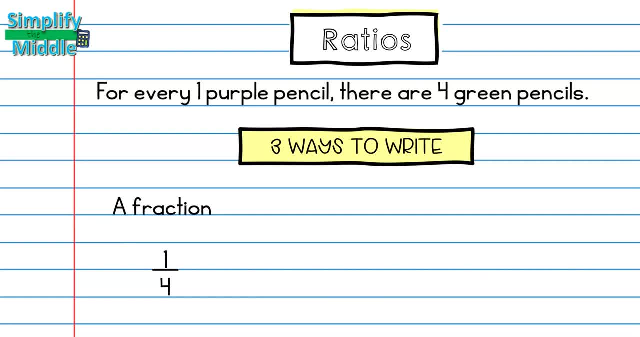 green. Another way to rate a ratio is using the word two, So there are one to four: purple to green pencils. The last way of rating a ratio is with a colon. We also say this as two, So this is also one to four. 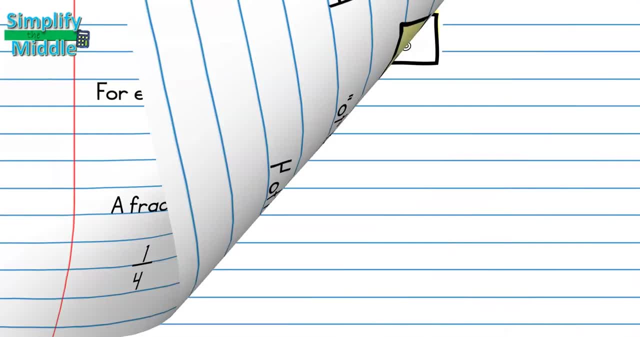 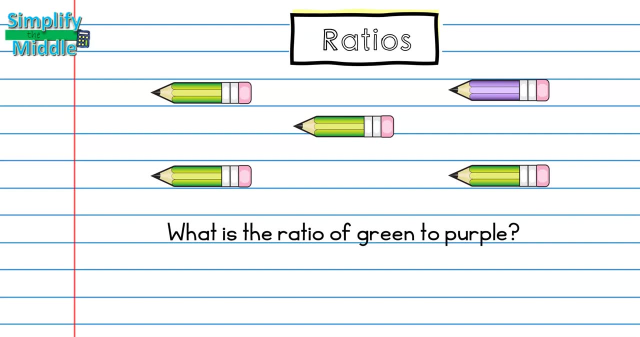 Let's take a look at another example. We're still going to use the same pencils from the last example, but this time the ratio asks for the number of green to purple. I still have four green and one purple, So when I write my fraction, I need to write what came first in the ratio, as 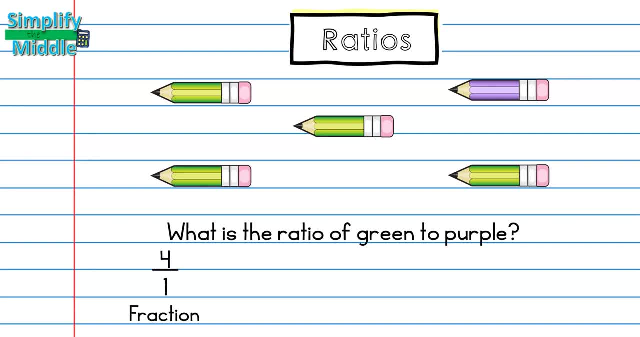 the numerator. So I have a numerator of four which represents my four green, and a denominator of one which represents my one purple. You might be asking yourself: can I simplify the number four over one to just four? And the short answer is no. We do not write a ratio as a whole or a mixed number, because we are 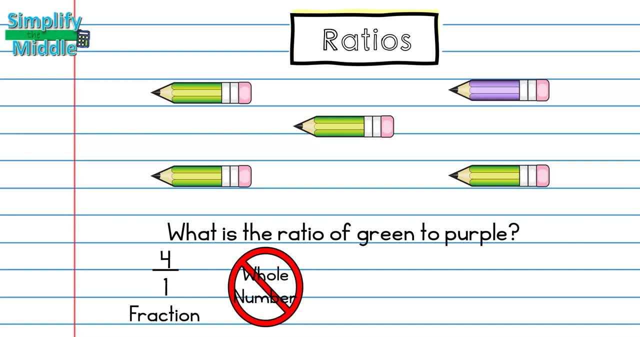 comparing two items and need to show two numbers that describe our items. We never write an improper fraction as a mixed number. for this reason, The next way of writing the ratio is with the word two. So we have four to one, green to purple, and then colon is going to be the.